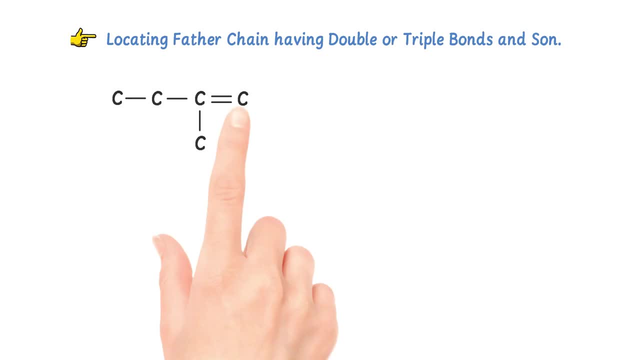 the other hand, 1,, 2,, 3,, 4.. There are also 4 carbons present in this chain, but there is one double bond present in it. So this is the father chain and this carbons. Now 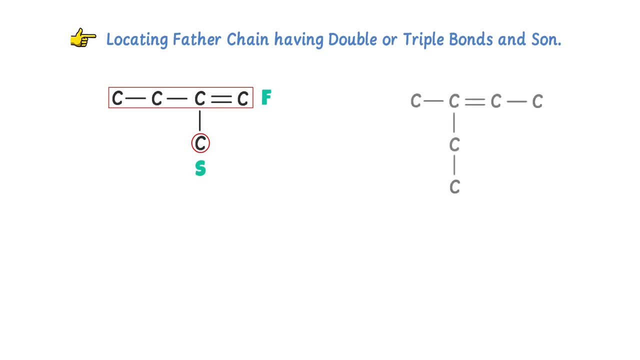 we will locate the father chain and the son: 1,, 2,, 3,, 4.. There are 4 carbons and one double bond present in this chain of carbon. Let me try one another chain: 1,, 2,, 3,, 4,, 5. There. 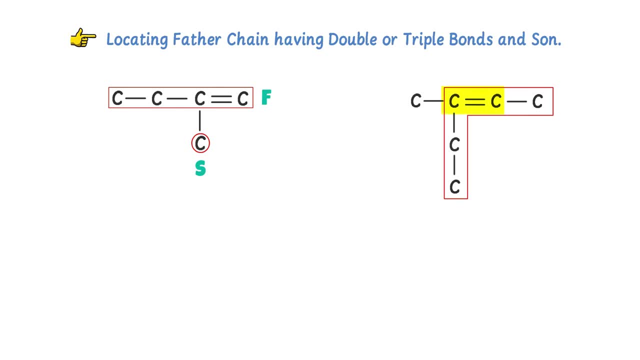 are 5 carbons and one double bond present in this chain. So this is the father chain and this carbon is his son. Thirdly, consider this organic compound. We will locate the father chain and his son: 1,, 2,, 3,, 4, 5.. There are 5 carbons present in this chain, but it 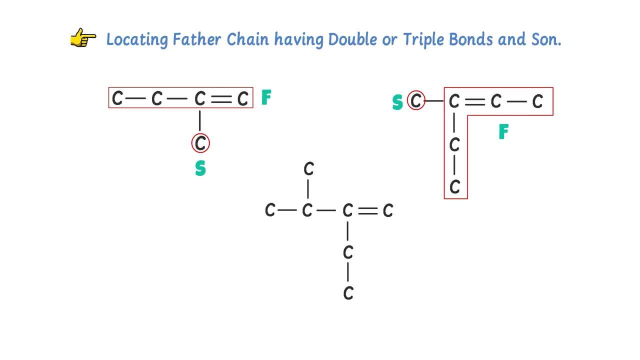 has no double bond, Hence I skip it Now. 1,, 2,, 3, 4.. There are 4 carbons and one double bond present in it. So this is the father chain and this carbon. Let me try one another. 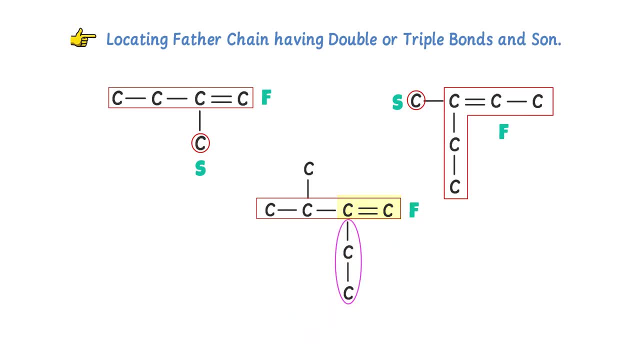 chain: 1, 2,, 3, 4.. There are 4 carbons and one double bond present in it. So this is the father chain. These 2 carbons are his son's and this one carbon is his son. Fourthly, 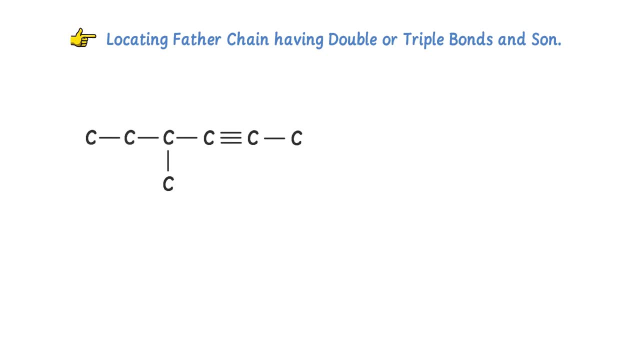 consider this organic compound. We will locate the father chain and son 1,, 2,, 3,, 4,, 5.. There are 5 carbons and one triple bond present in this chain. Let me try one another chain. 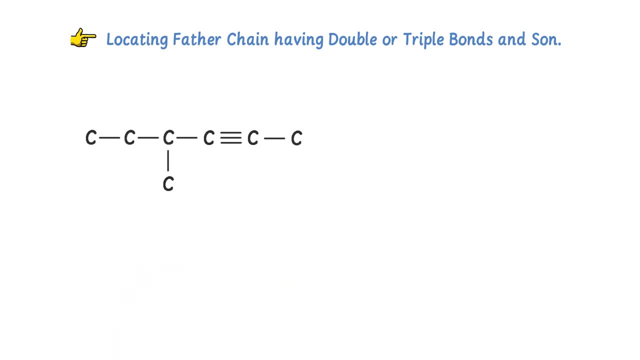 1,, 2,, 3,, 4,, 5, 6.. Hear this in this description: 1, 2,, 3,, 4, 5.. There are five carbons and one. There are six carbons and one triple bond present in it. 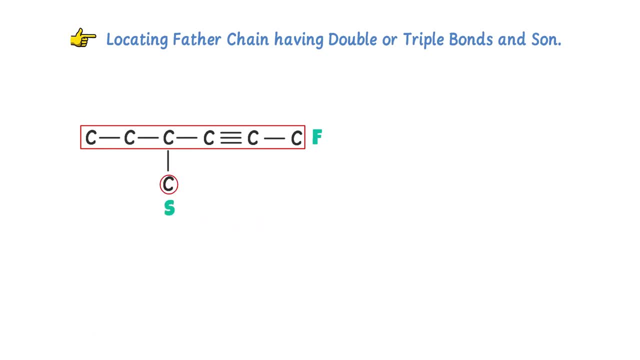 So this is the father chain and this is his son. Finally, consider this organic compound. We will locate the father chain and his son. One, two, three, four, five. There are five carbons and one triple bond present in it. 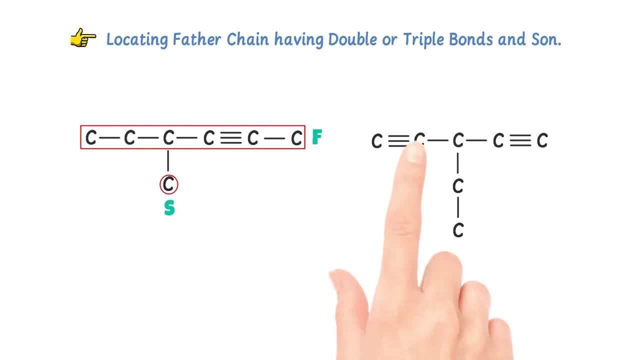 Let me try one another chain: One, two, three, four, five. There are also five carbons present in this chain, but there are two triple bonds present in it. So this is the father chain and these two carbons are his sons. 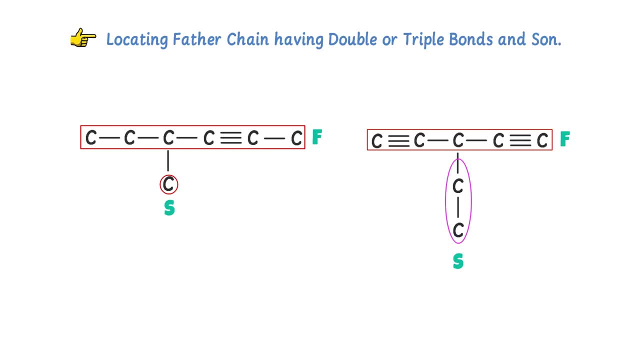 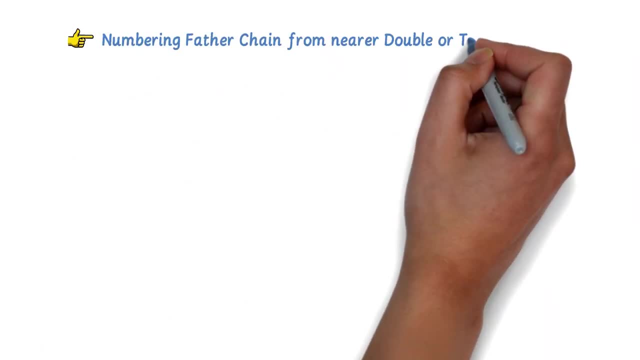 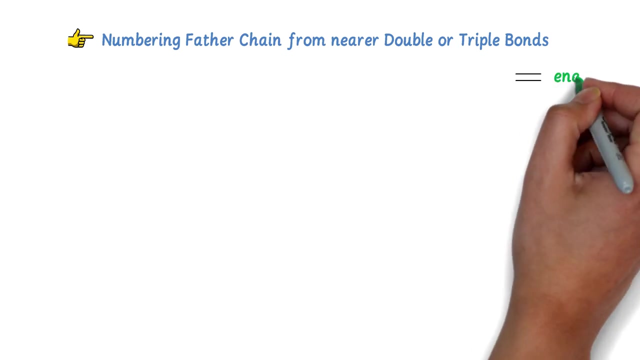 Thus, by this way, we can locate the father chain and his son. Now let me teach you the second rule. The second rule is numbering the father chain from where double or triple bonds are nearer. Remember that for double bond, we write IN, and for triple bond we write IN. 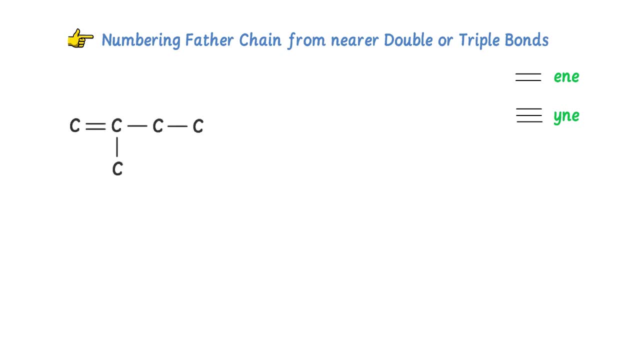 For example, consider this organic compound. I locate the father chain and his son: One, two, three, four. This is the father chain and this is his son. Now listen carefully. I number the father chain from both the INs. 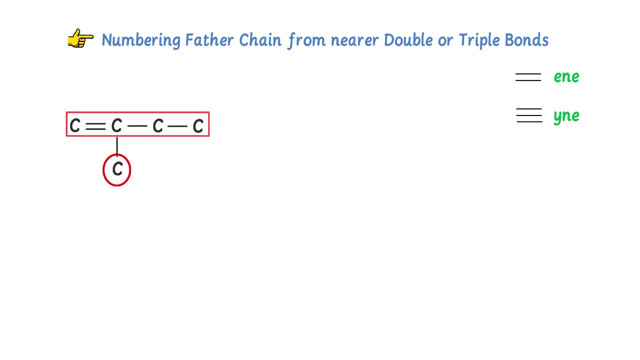 Let me repeat it. I number the father chain from both the INs Like one, two, three, four. also one, two, three, four, According to this order of numbering. the double bond is present in the third carbon. 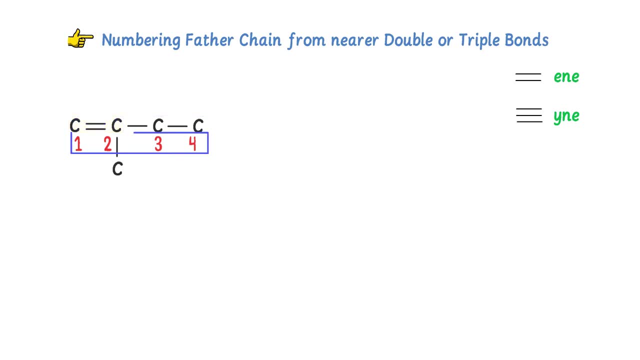 So I skip this order of numbering, While according to this order of numbering, the double bond is present in first carbon. So I select this order of numbering. Now I will name the father chain and the son. There are four carbons present in the father chain. 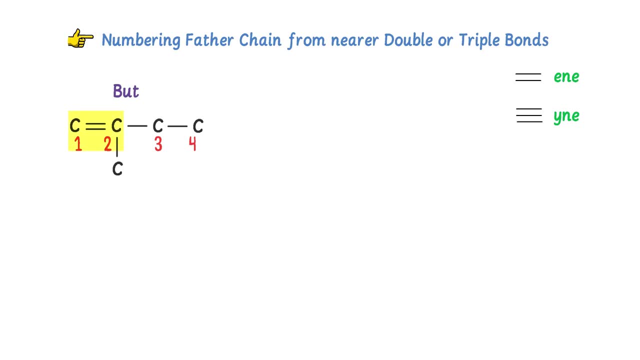 I write BUTE. Also, there is one double bond I write IN: The double bond is present at first carbon. I write ONE. So the father chain is ONE BUTE IN. Remember that some people write it as BUTE ONE IN, which is also correct. 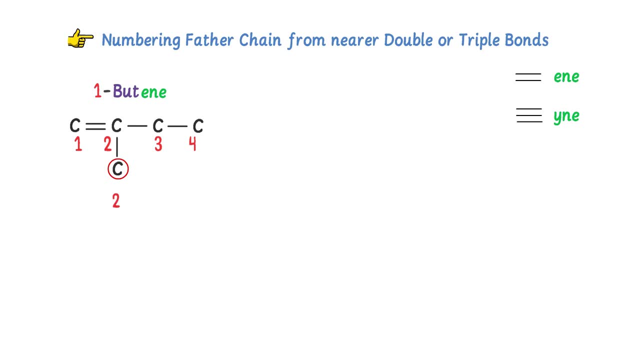 Now the son is present. at second position I write TWO. There is only one carbon. I write TWO METHYL As a convention. firstly I write the son's part and then I write the father's part. TWO hyphen METHYL. hyphen ONE: hyphen BUTE IN. 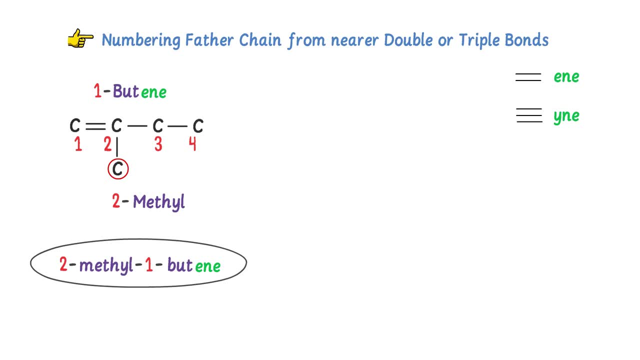 So the name of this organic compound is TWO METHYL ONE BUTE IN. Secondly, consider this organic compound. I select the father chain and son ONE, TWO, THREE, FOUR, FIVE. So this is the father chain and this is his son. 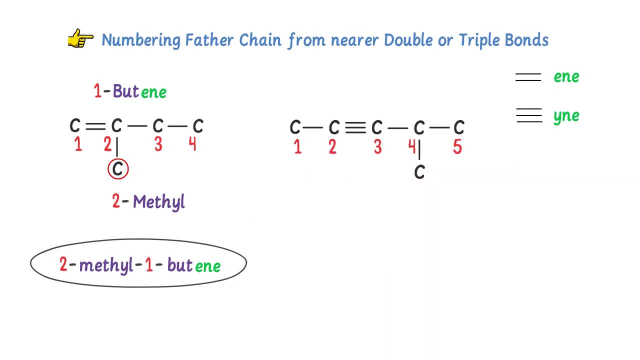 I number the father chain: ONE TWO, THREE FOUR FIVE. Also ONE TWO THREE FOUR FIVE. According to this order, the triple bond is present at third carbon. I skip this order, While according to this order, the triple bond is present at second carbon. 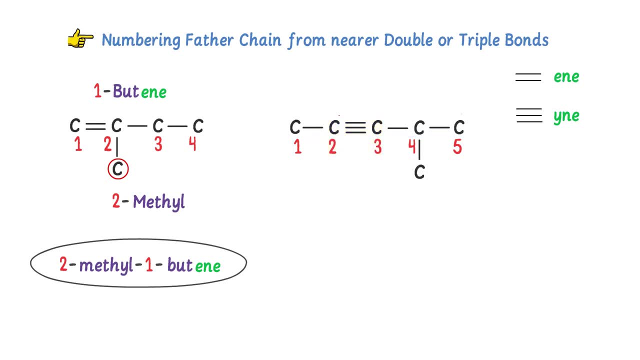 I select this order of numbering. I name the father's part and the son's part. The triple bond is present at second carbon. I write TWO. There are five carbons present in the father chain. I write PENT. Also, there is one triple bond present in the father chain. 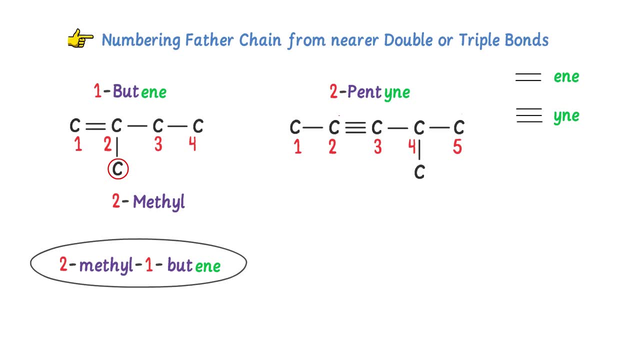 I write EIN. So the father part is TWO PENT EIN. What about the son's part? Well, it is present at the fourth carbon. I write FOUR METHYL. Now I combine the son's part and the father's part. 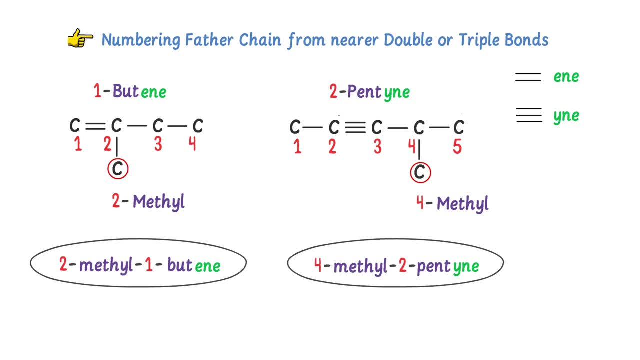 FOUR METHYL TWO PENT EIN. Thus, the name of this organic compound is FOUR METHYL TWO PENT EIN. Thirdly, consider this organic compound ONE, TWO, THREE, FOUR, FIVE. This is the father chain and this is his son. 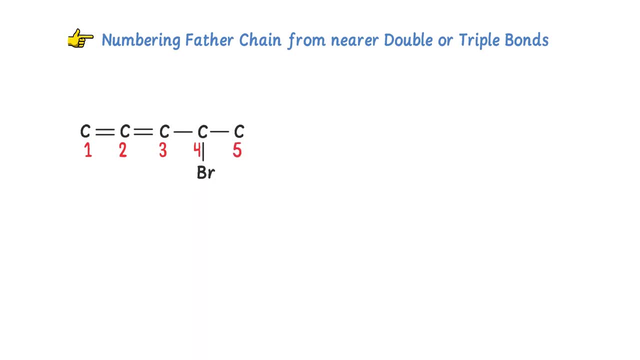 I number the father chain: ONE TWO, THREE, FOUR FIVE. Also ONE TWO, THREE FOUR FIVE. I select this order. We can see that in the father chain there are two double bonds present. Note it down that when there are two double bonds present in the father chain, we use 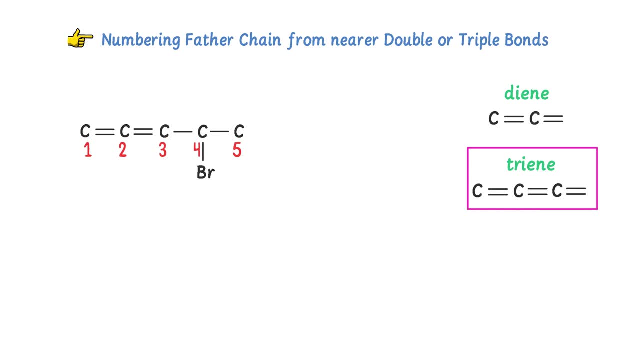 DIENE and we use TRIENE for three double bonds. So there are five carbons present in the father chain. I write PENTA. For the two double bonds I write DIENE. One double bond is present at first position and the another double bond is present at 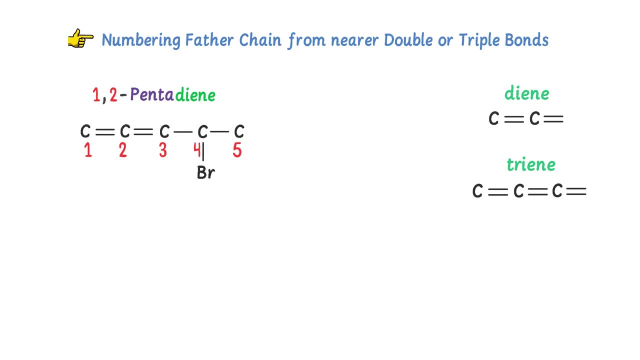 the second position. So the father chain is ONE COMMA TWO, HYPHEN, PENTA DIENE. What about the son's part? Well, it is FOUR BROMO. Thus we get FOUR BROMO, ONE COMMA TWO, PENTA DIENE. 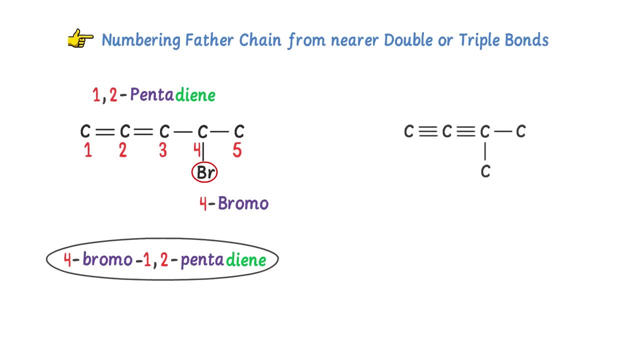 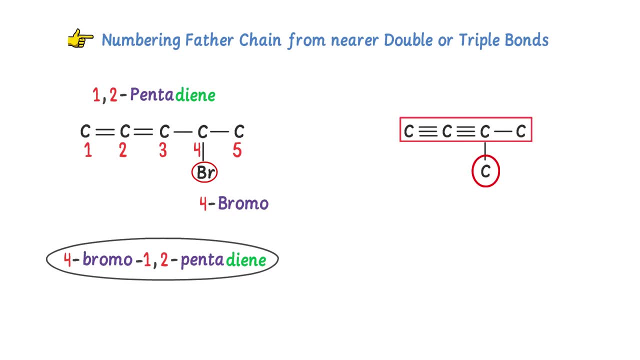 This is the father chain And this is his son. I number the father chain: ONE TWO THREE FOUR. Also ONE TWO THREE FOUR Because triple bond is nearer. according to this order of numbering And the father chain, There are FOUR carbons. 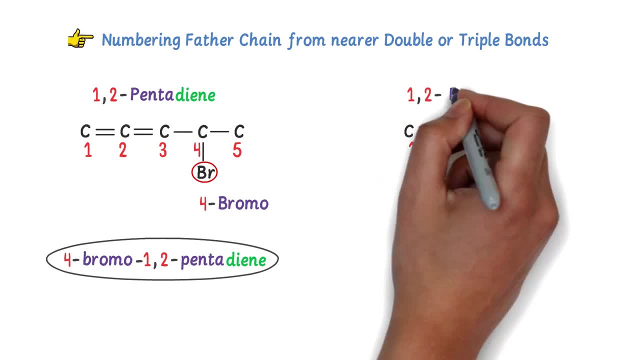 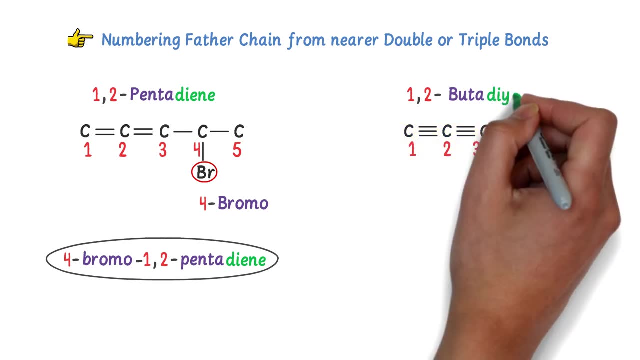 It is the third one. I write 1,2-buta. also, there are two triple bonds present in the further chain. I write diene, So I get 1,2-butadiene. The sun is located at the third position. 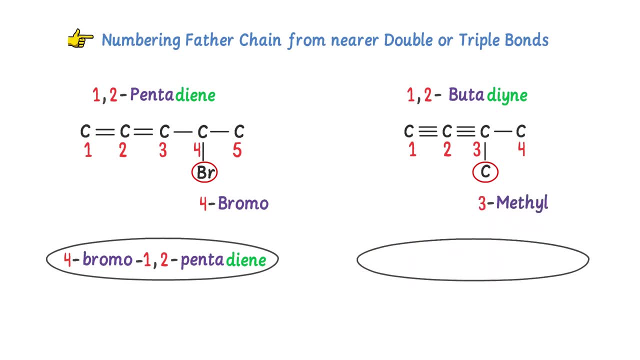 I write 3-methyl, So I get 3-methyl-1,2-butadiene. Finally, consider this organic compound. I look at the father chain and son: 1,2,3,4,5.. This is the father chain and this is his son. 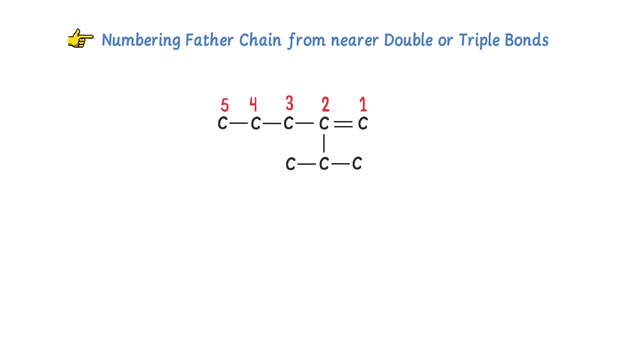 I number the father chain 1,2,3,4,5.. In the father chain there are 5 carbons and 1 double bond. I write 1-pentene. In the son's part there are 3 carbons. 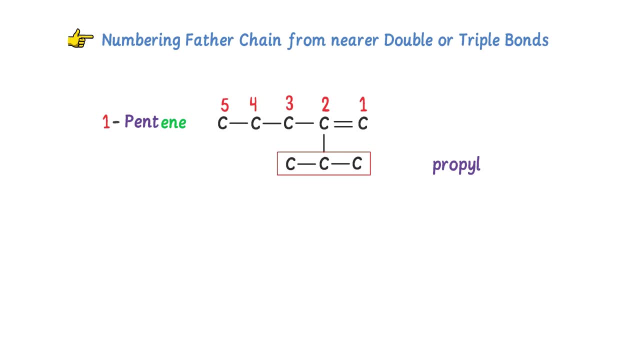 I write propyl. These 3 carbons are 1,2-butadiene. In the case where the Keeper and the naturopath are branched, I write iso. It is present. at the second position, I write 2, so I get 2-isopropyl-1-pentene. 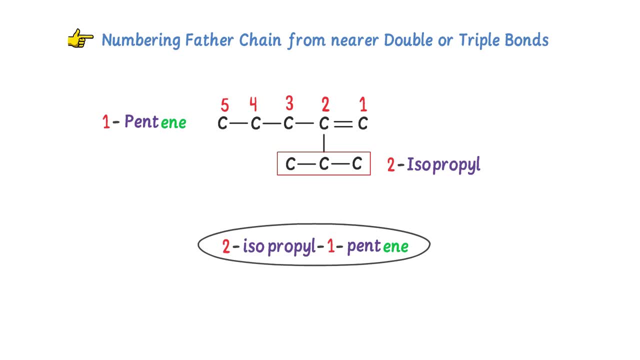 Thus, this is the second rule through which we can name the father's part and the son's part. the third and the last rule is: in case of double and triple bonds, the nearer bond is selected for numbering organic compound. This is the father chain. this is the son. I number the father chain. 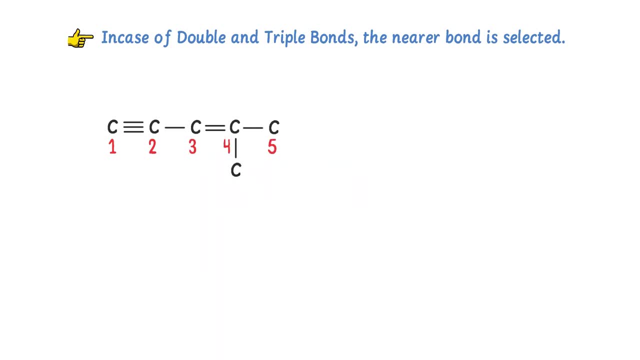 1,2,3,4,5, also 1,2,3,4,5.. According to this order, the double bond is present at second position and the triple bond is present at the fourth position According to this order. 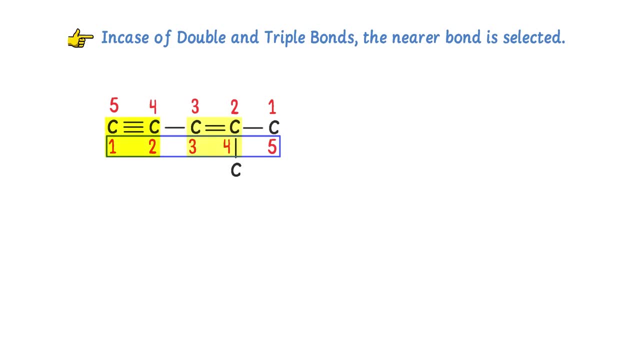 the triple bond is present at first position and the double bond is present at third position. So I select this order of numbering because triple bond is nearer. according to this order of numbering Now there is een part of alkene and ein part of alkyne in the father chain. 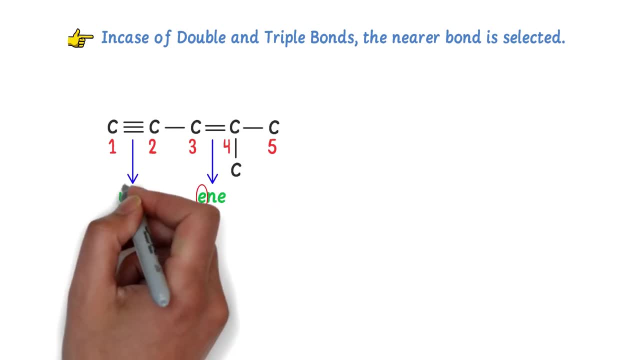 According to alphabetic order, e comes first, then y, So we will write een part and then we will write ein part. There are five carbons present in the father chain and the double bond is present at the third position. I write 3-pentene. Now I remove this e from pentene. The triple bond is present. 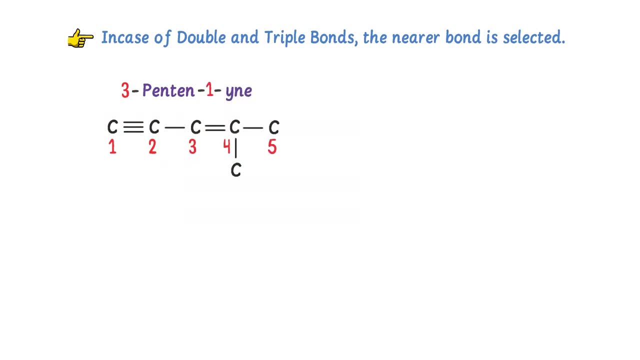 at first position I write 1-ein. Now the son is 4-chloro. Thus I get 4-chloro 3-pentene 1-ein. This is the name of this organic compound. Subtitles by the Amaraorg community. 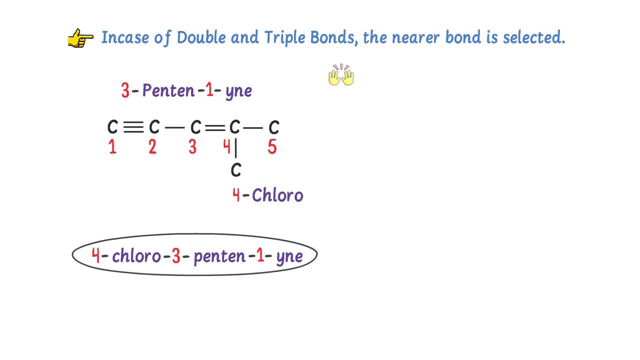 Lastly, let me teach you one exceptional case. If the double and triple bonds are present at the same position, select the double bond for numbering. For example, consider this organic compound: This is the father chain and this is his son. I number the father. 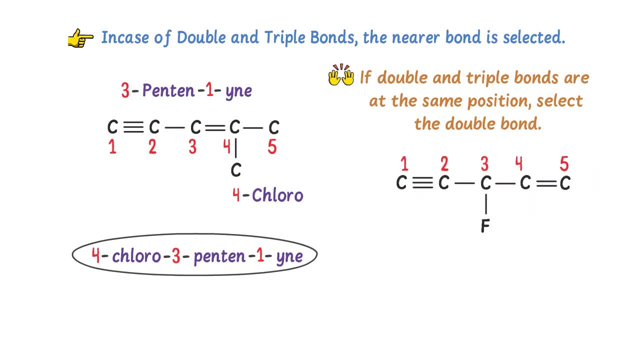 chain: 1, 2,, 3,, 4, 5.. Also 1,, 2,, 3,, 4, 5.. Now, according to this order of numbering, the double bond is present at first position.